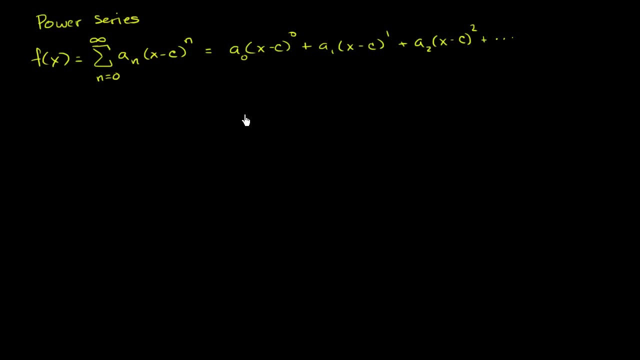 on an easier to operate on function. And this shows up in electrical engineering and it shows up even in finance. In bond trading, bond traders will actually use a power series approximation to figure out what a bond's price might do or what the corresponding implied interest rate on a bond. 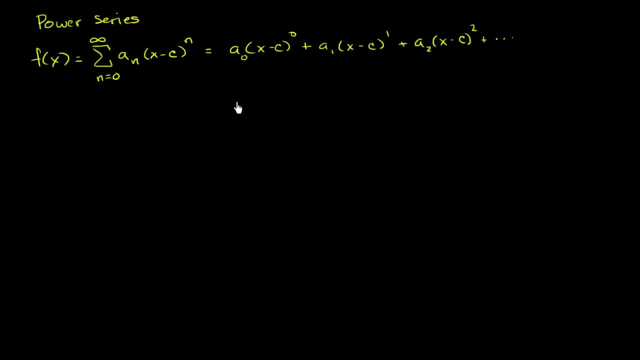 might be, But we're not going to worry about that right now. We're just going to deal with it a little bit more mathematically. Now, the one thing that you might see when you look at this well isn't a geometric series where 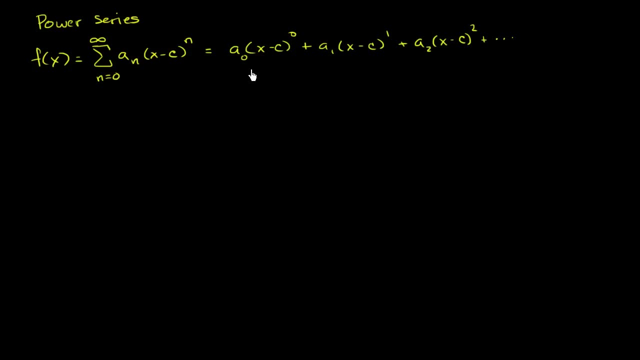 if I make the common ratio x, isn't that a special case of a power series? And you would be correct in assuming that. So let's write down a geometric series where the common ratio is x, So geometric series. So let's define a function g of x as a geometric series. 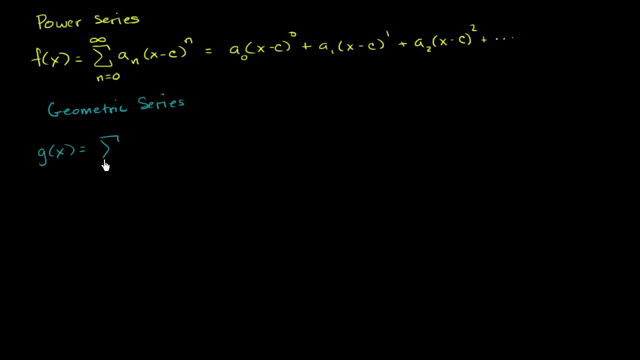 where the common ratio is x instead of the r that we're more typically used to represent the common ratio. So n equals 0 to infinity, of a times x to the n. So what's the difference between these two things? Well, this is just a special case. 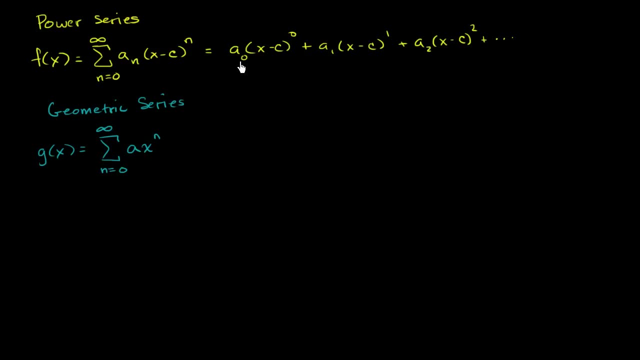 We're making c equals 0. And we're making all of these a sub 0, a sub 1, a sub 2, they're all just going to be equal to a, And we know that we can expand this out as a times x to the 0 plus a times x to the first power. 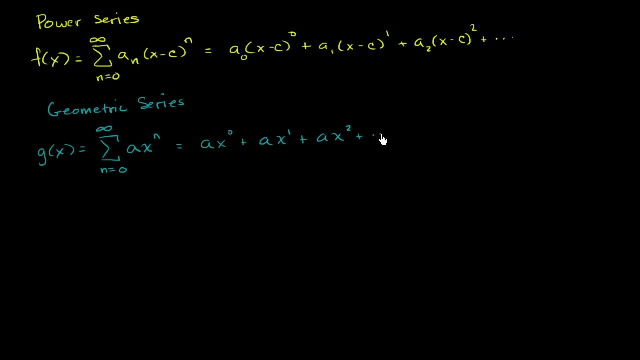 plus a times x squared, And we just go on and on and on forever. This is an infinite series. Well, we've already seen How we can take this sum. In fact, we've already done multiple examples where we take sums of infinite series. 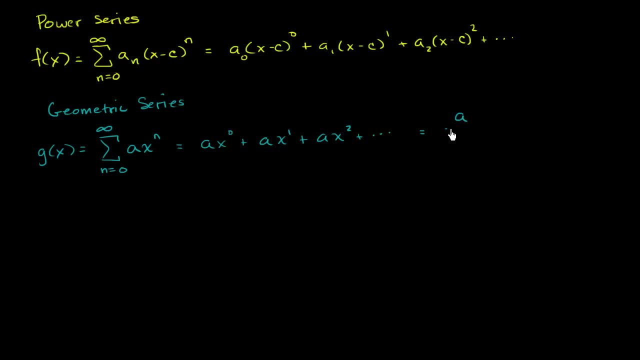 and we've derived the formula that gets us that this is going to be equal to a over 1 minus our common ratio, And in this case, our common ratio is equal to x. What's interesting about this is, instead of going from this geometric series expanded form, 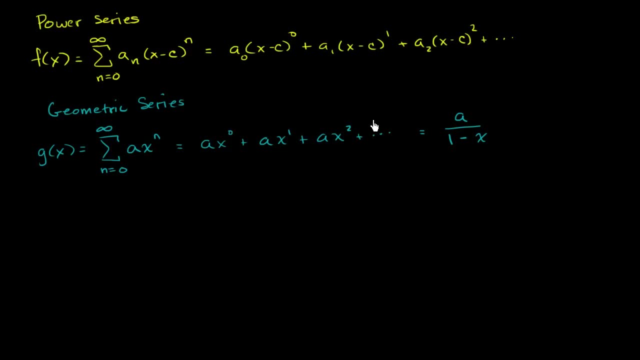 to what the sum needs to be. we can use this to go The other way. if we can get some functions into this form, we can then expand them out as geometric series, or essentially we will find their power series representation, Because a geometric series is a special case of a power series. 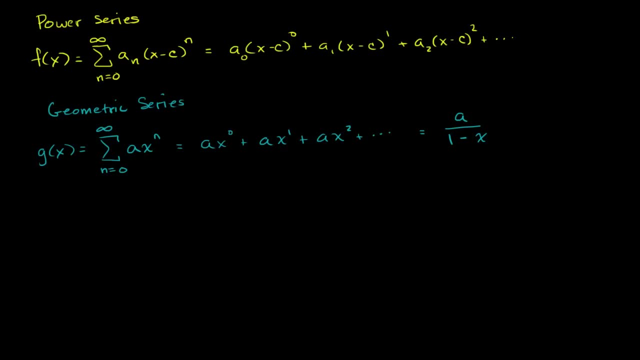 And to show an example of that, let's take the function h of x is equal to 1 over 3 plus x squared. So I encourage you now to pause this video and try to rewrite this function in this form right over here. 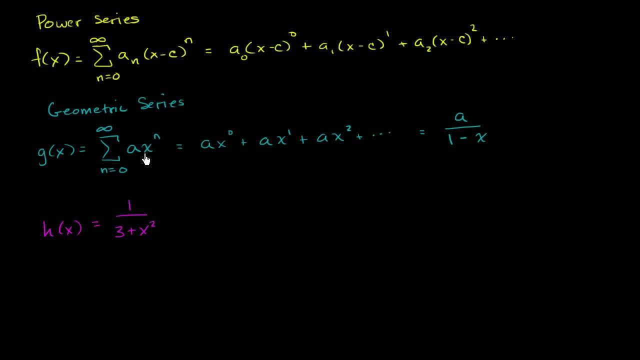 And if you can write it in this form, to then go and write it as a geometric series. So I'm assuming you've given a go at it, So let's try to do it. So we want a 1 right over here. 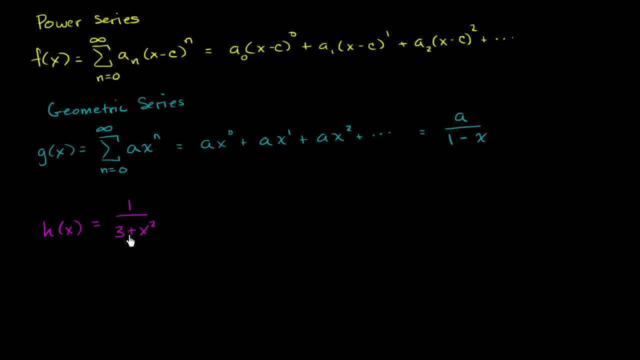 And we want to subtract something. So if we want a 1 right over here, let's divide the denominator by 3.. So this is equal to, or let's factor out a 3, I should say 1 over 3 times 1 plus x squared over 3.. 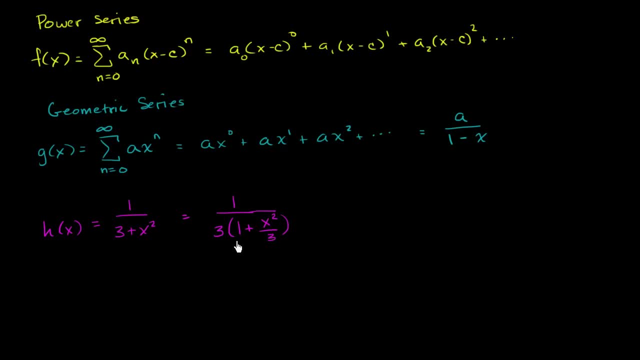 All I did here is I factored out a 3.. I divided 3 by 3, factored it out, And then I factored out a 3 from x squared. So if I were to redistribute, you would get this again. 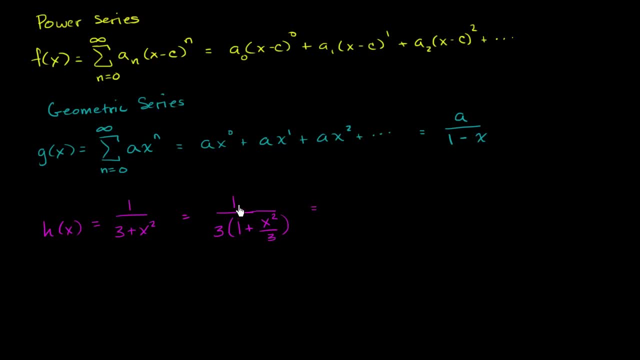 Now I could rewrite this as: instead of 1 over 3, I could write this as: let me write it this way: I could write it as: so this part right over here I could write it as 1 third over 1.. 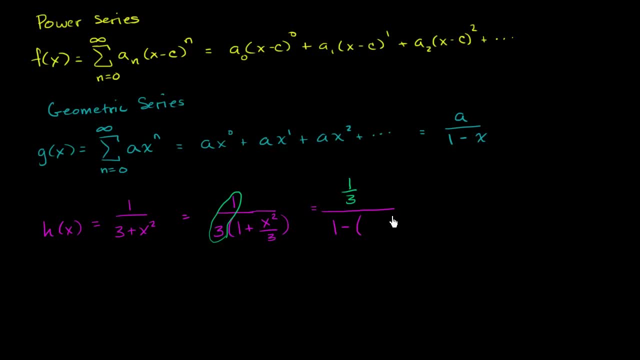 And I want to subtract this thing instead. So 1 minus, and I could write negative x squared over 3.. Notice: adding x squared over 3 is the same thing as subtracting negative x squared over 3.. So now I've written in this form: 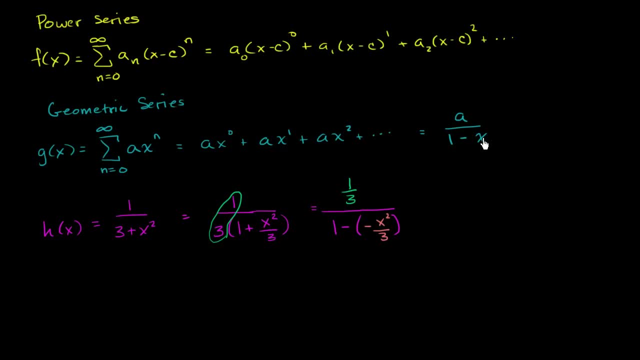 I have my a. My a would be 1, third, And then my common ratio x is going to be negative, x squared over 3.. So now I can rewrite h of x. I can say that h of x is going to be. 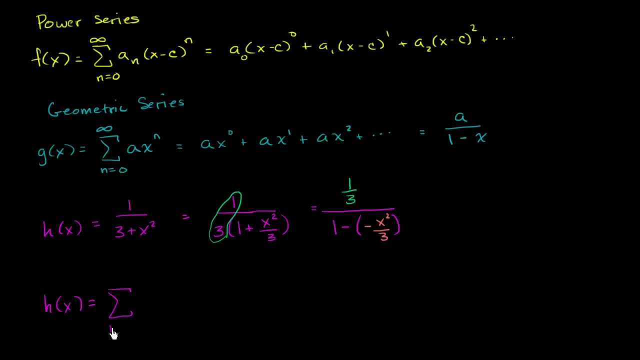 equal to the infinite series. So I'll go from n equals 0 to infinity. My a is 1 third, and then my common ratio is negative x squared over 3.. Negative x squared over 3, I'm going to raise that to the nth power. 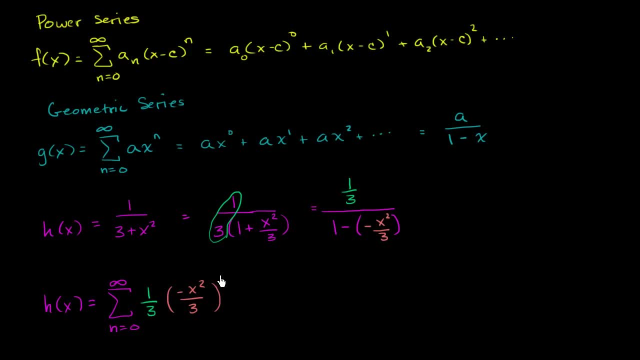 And so if I wanted to expand it out- and actually maybe I'll write that in purple, If I wanted to expand this out, what would it look like? Well, this would be equal to well, the first term when n is equal to 0, this whole thing just becomes 1.. 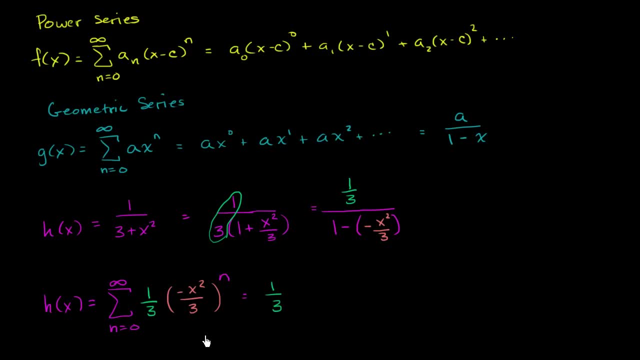 So this is just going to be 1 third And then the next term. I'm just going to multiply by the common ratio. I'm going to multiply. I'm going to multiply by negative x squared over 3.. So this is going to be equal to negative. 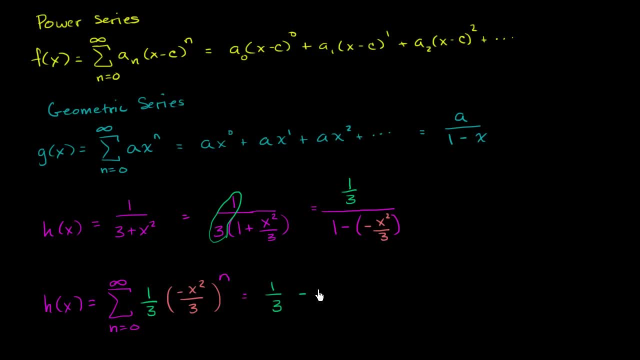 So if I take 1 third and multiply by negative x squared over 3, that's going to be negative x squared over 9.. And then if I were to multiply by negative x squared over 3 again, well, now I'm going to get positive x. 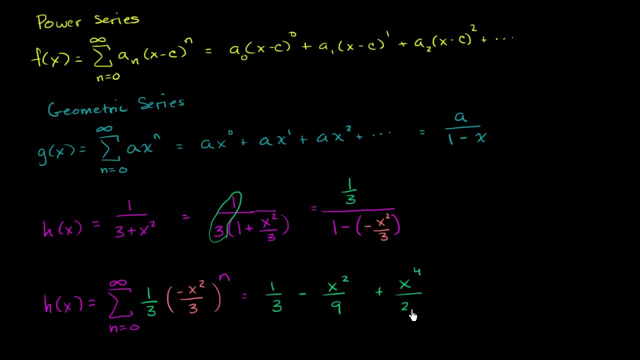 to the fourth over 27.. Notice the common ratio: Every time, to go from here to there, I have to multiply by negative x squared over 3.. To go from there to there, I have to multiply by negative x squared over 3.. 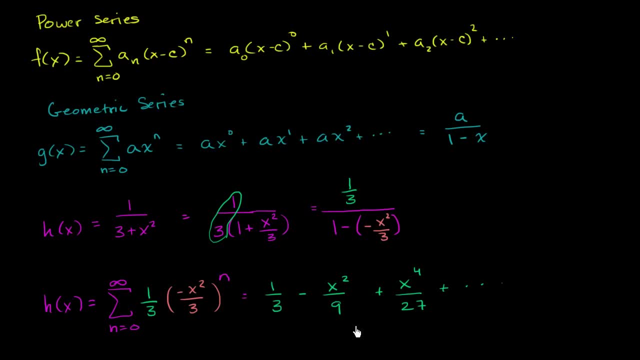 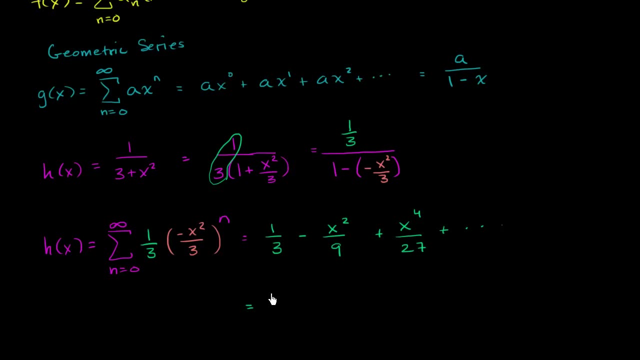 And I could keep going on and on and on. And if I really wanted to write it in that form, I could just let me make this a little bit clearer. So I could just write it, as I could just write this as 1 third minus 1 ninth times x squared: 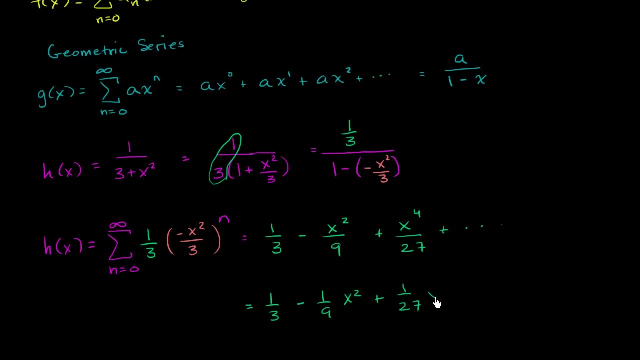 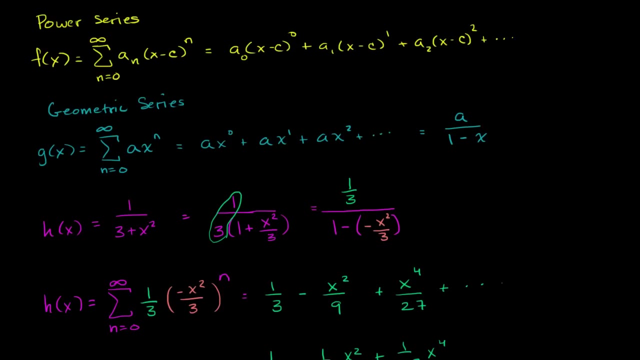 Plus 1, 27th times x to the fourth, And you might say, well, this is almost the same form, But these forms up here we had right. here you just have the x to the 0 term and then the x squared term. 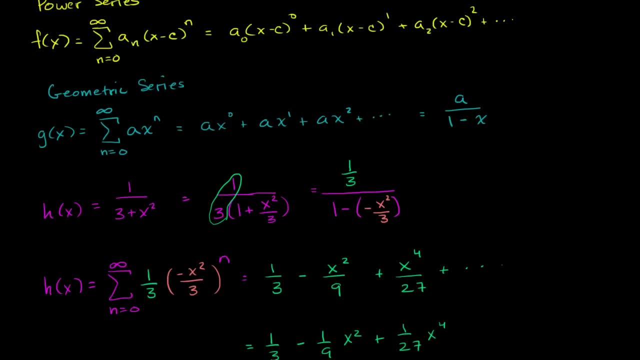 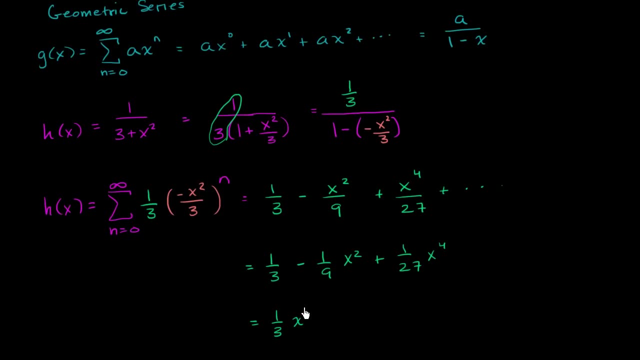 What about this? Well, remember, you could just make this coefficient 0. So I could even rewrite it like this: I could say: this is equal to 1 third times x to the 0, plus 0 times x to the first power. 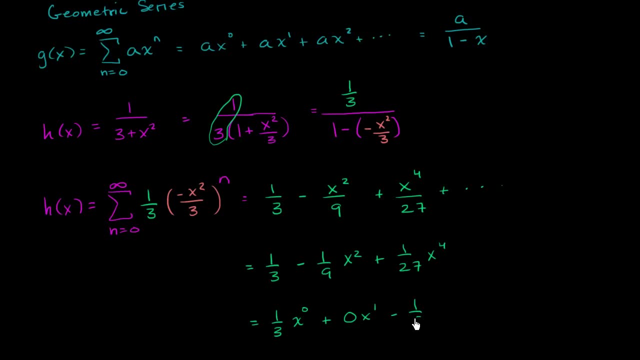 plus 1.. Or let me write this: minus 1 ninth x squared, And then plus 0 times x to the third power, And then plus 1 over 27 times x to the fourth power, And then notice I have this in the exact same form. 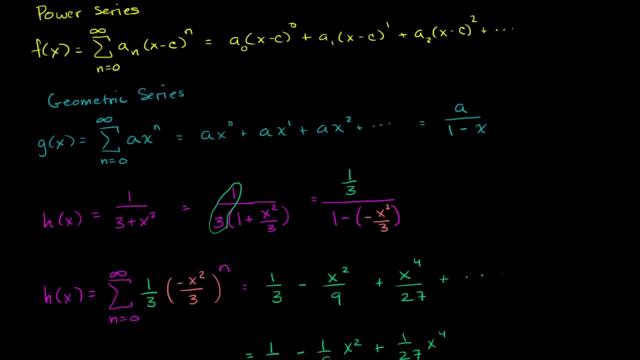 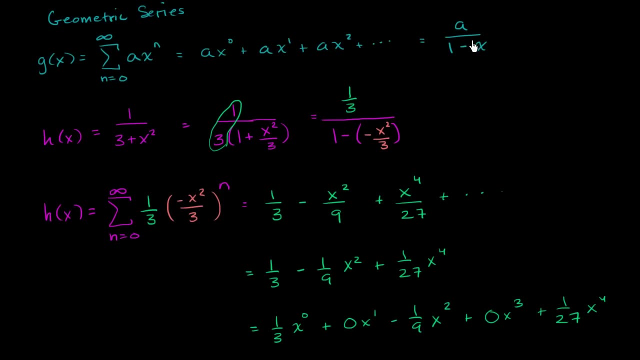 I have the exact same form as our original power series. So, without using any calculus, we were able to take a function like this, represent it like this and then find a power series representation for it, And I would this one. I don't want to confuse you here.